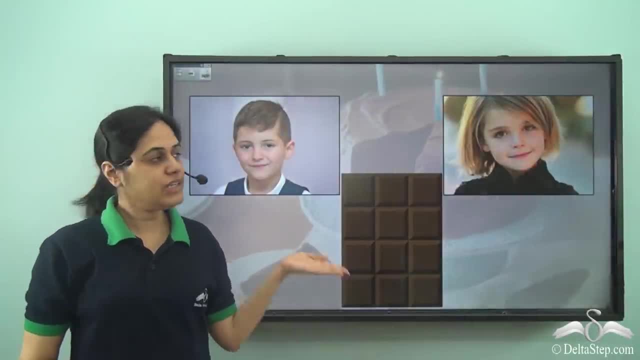 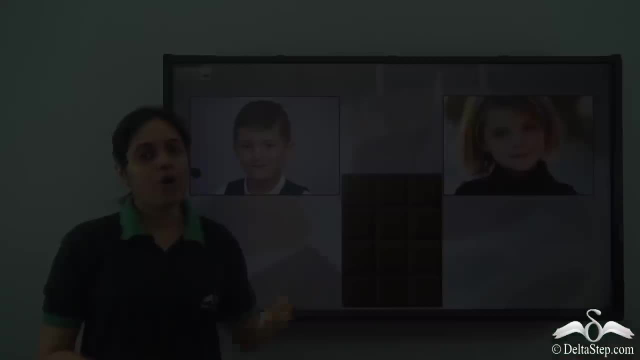 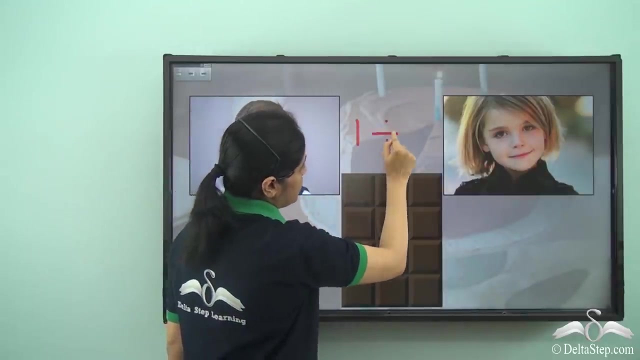 Now what would she do? So there is just one chocolate, but there are two kids. So will she give it to Abeer? That wouldn't be fair, right? Or will she give it to his sister? That wouldn't be fair too. So now this one chocolate has to be divided in these two kids. 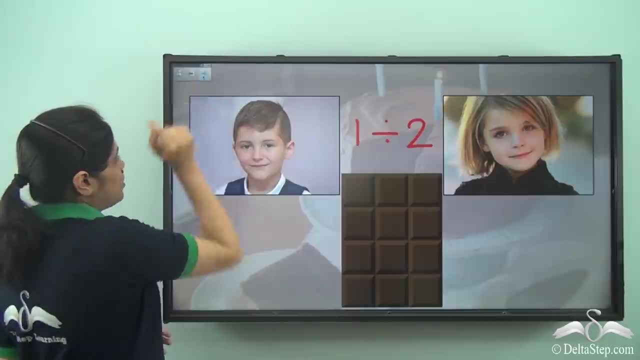 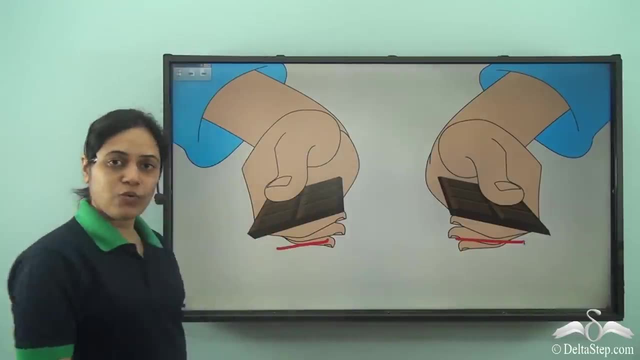 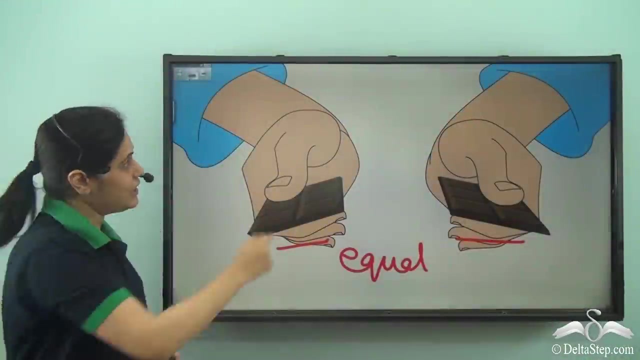 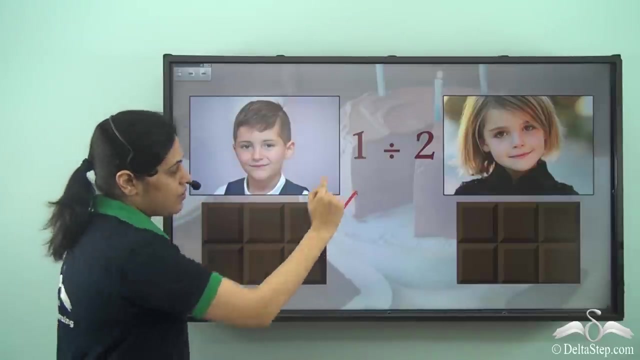 kids. So what does the mother do? She breaks the chocolate into two equal parts. So one, two equal parts. So, as we can see, she breaks the chocolate into two equal parts and gives one part to each of the two kids. So he gets one part and she gets one part. and this is 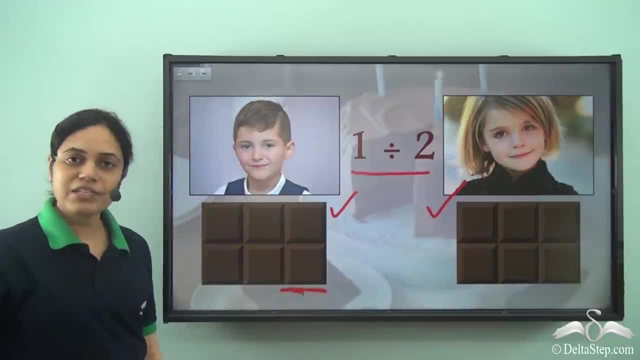 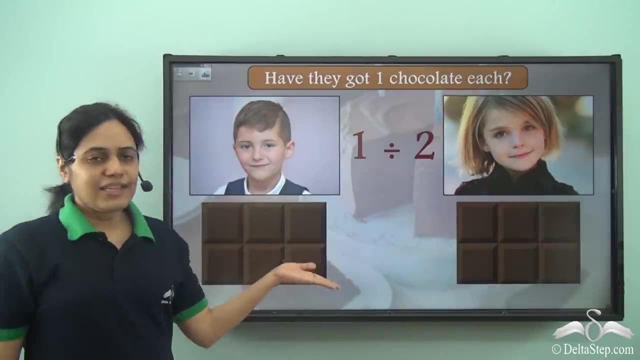 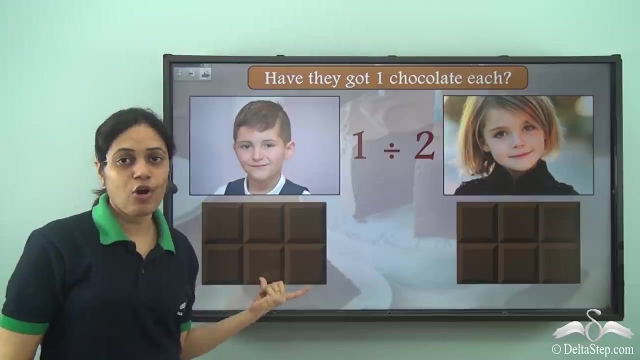 one divided by two. So this part is one divided by two, and even this part is one divided by two. So will you say that they have got one chocolate each? No, they haven't got one chocolate each. They haven't got one chocolate each. 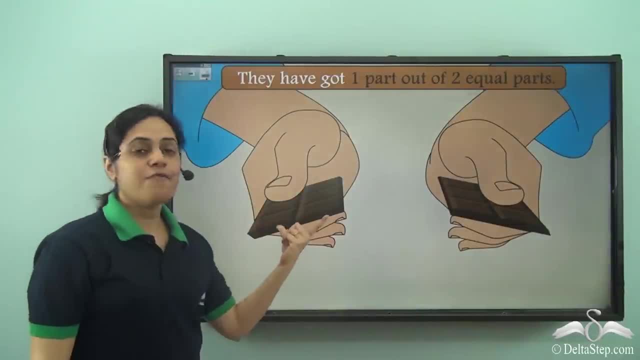 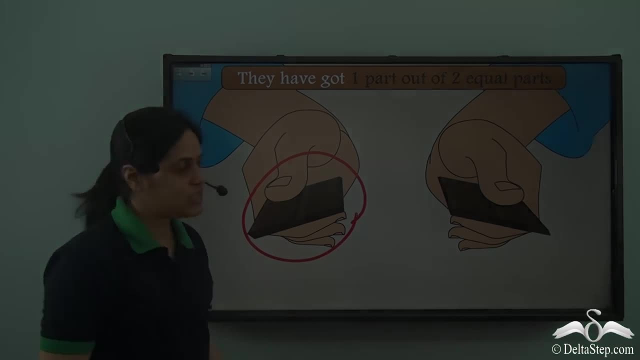 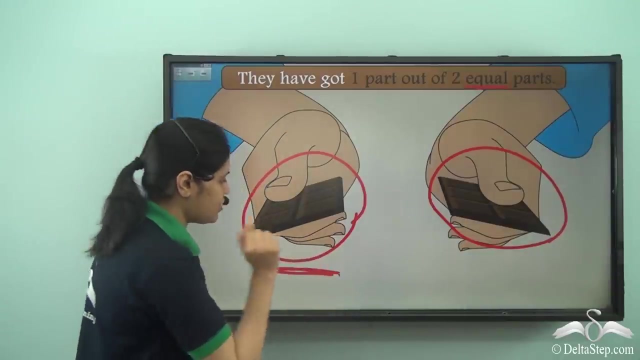 They have got an entire chocolate. What they have got is one part out of two equal parts. So Abir has got one part out of two equal parts. So his sister has got one part out of two equal parts. Now how do I write this part mathematically? I cannot write it one. 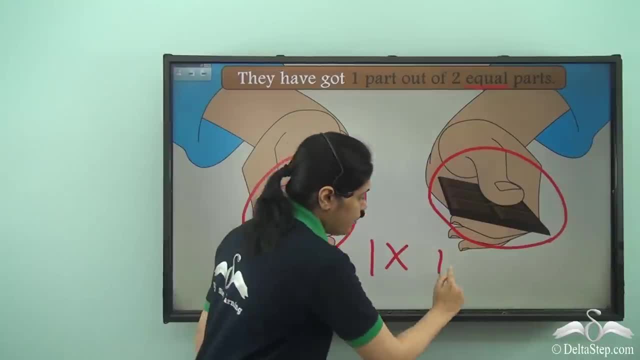 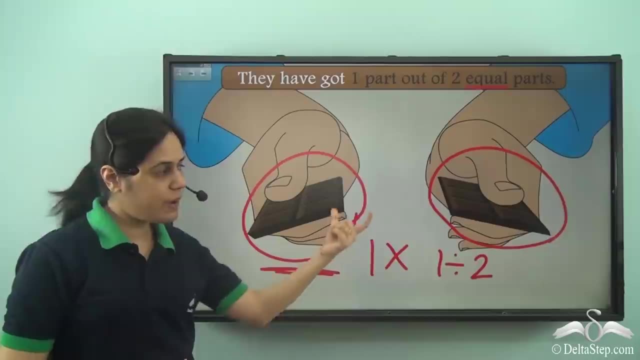 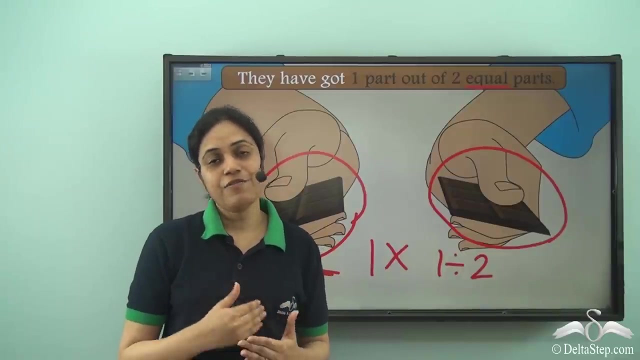 because it is not one, It is less than one. It is one divided into two equal parts. So this is one part out of two equal parts. This is one part out of two equal parts. So how do I write it mathematically? Well, we use fractions to write it mathematically, So let 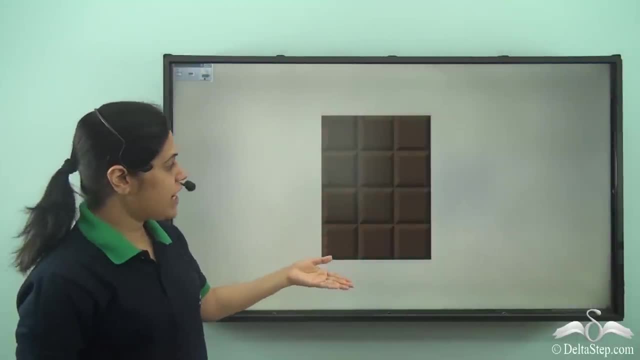 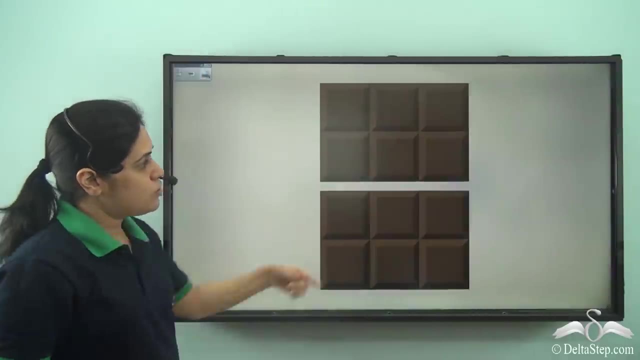 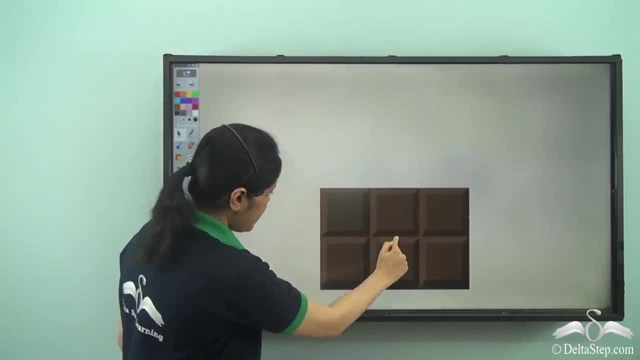 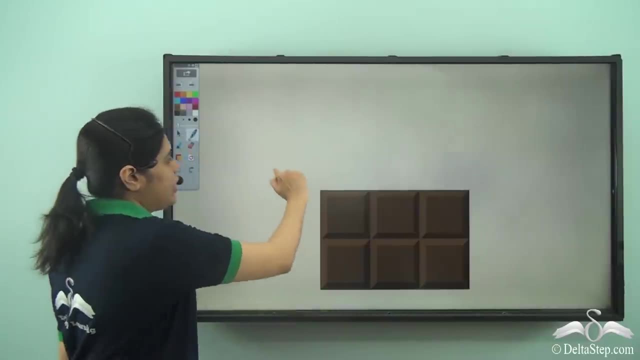 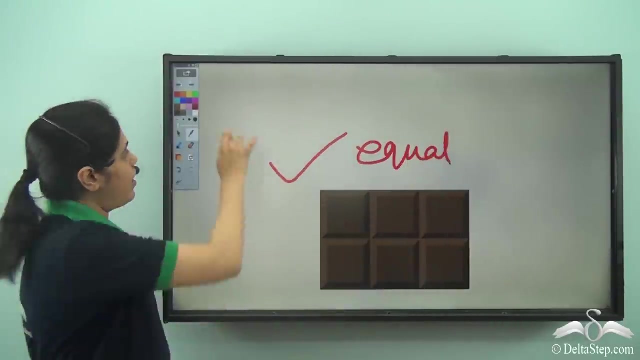 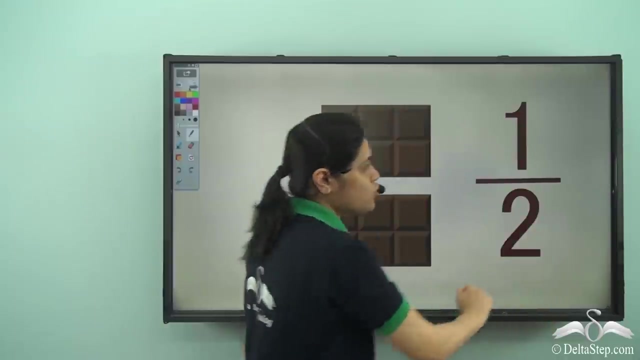 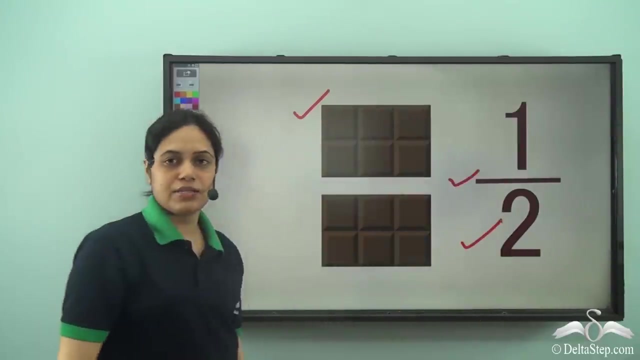 they are equal parts or not. So I take this and I overlap this on the second part and we see that they perfectly overlap. So the parts were equal and each of these parts can be written as 1 by 2.. So this part is one part out of two equal parts, Even this part. 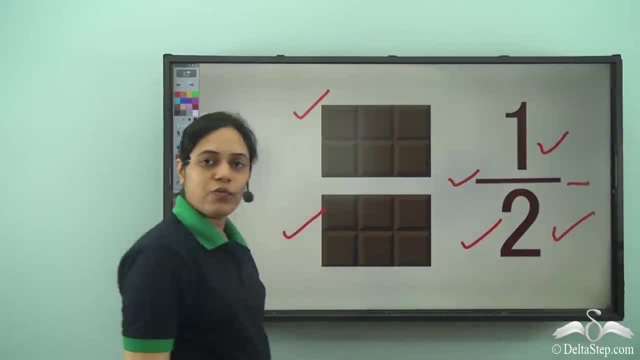 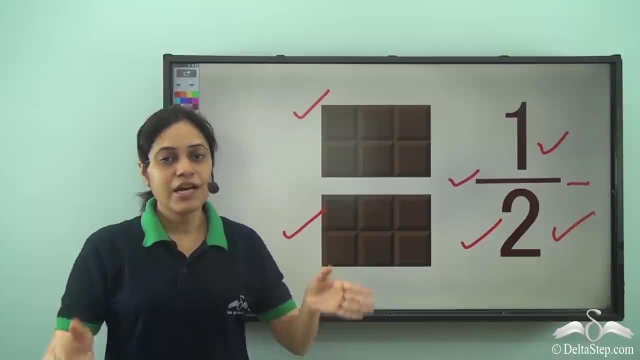 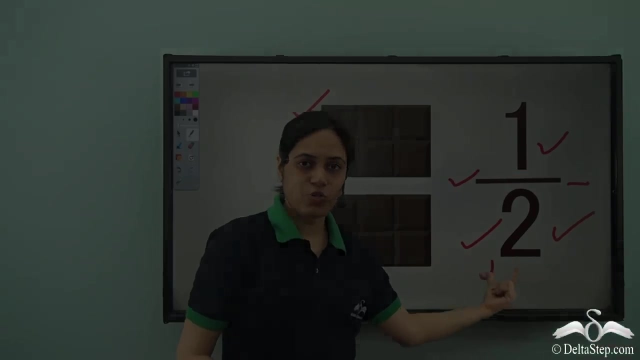 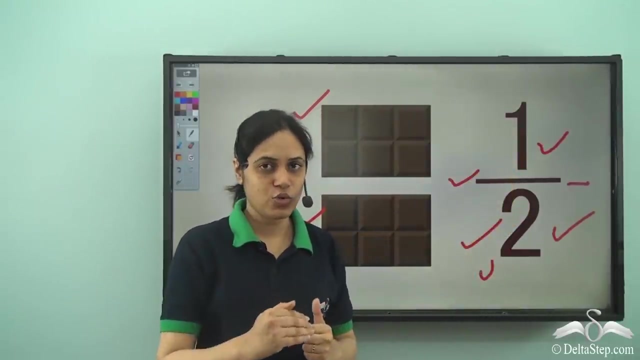 is one part out of two equal parts, So one out of two equal parts. So when the chocolate is divided into two equal parts, each part can be written as one- this line, and then two. We can read it as 1 by 2.. So 1 over 2, 1 and 2 and a line separating them. So this: 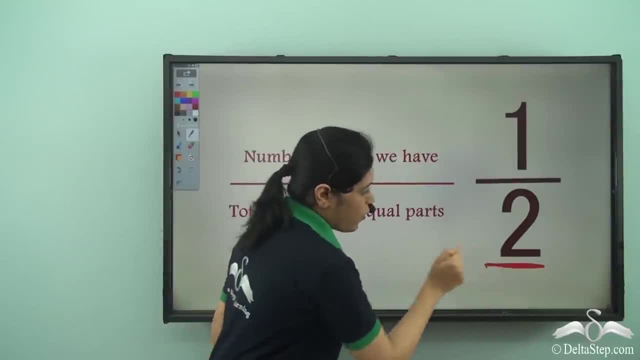 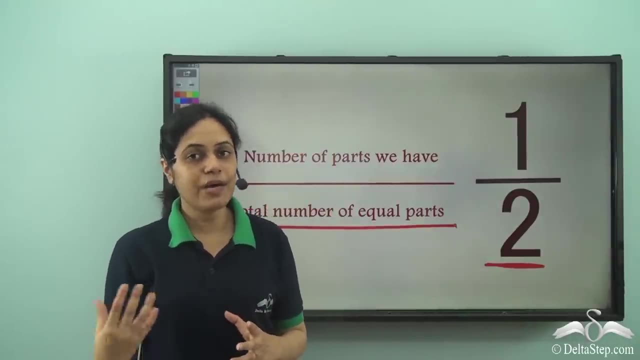 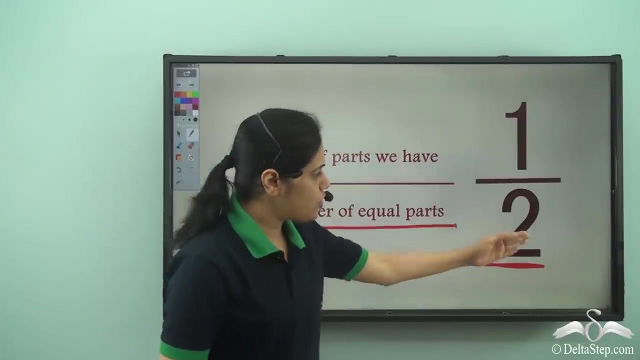 is how I write fractions. At the bottom I write total number of equal parts. So if something is divided into some equal parts, I write total number of equal parts. So the chocolate was divided into two equal parts, So I write 2 by 2.. 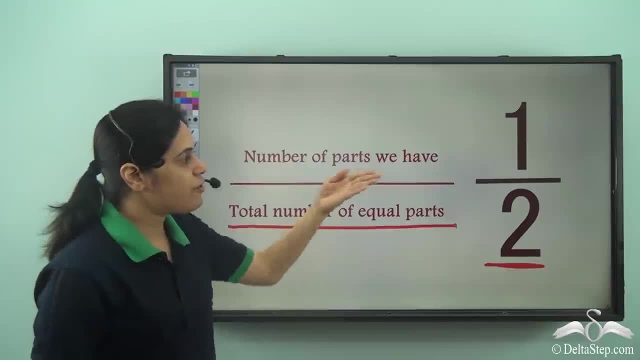 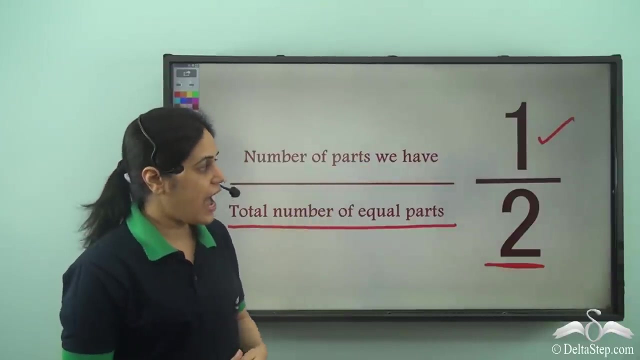 So let us write lower number to 2 and then a right two at the bottom, And number of rubber parts we have is written on top. So either of the two kids had one part, So one is written on top Number of parts we have. So we can say that each of the two kids had 1 by 2 chocolates. 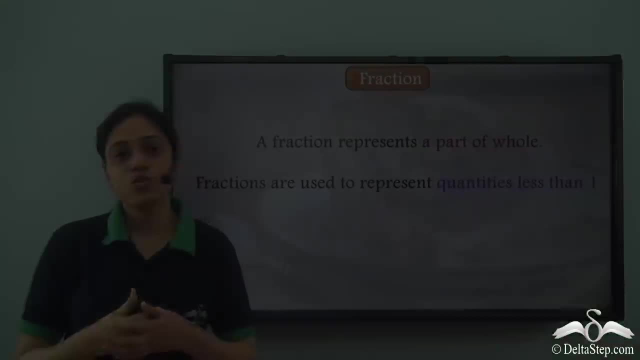 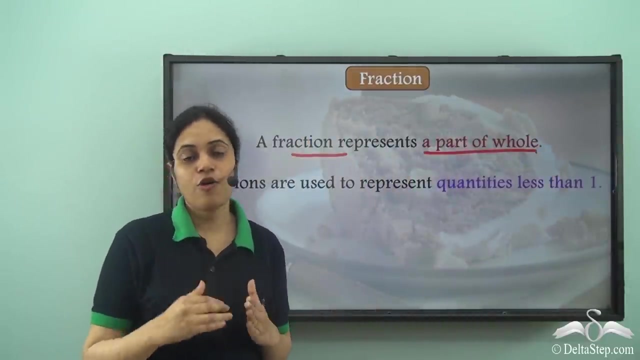 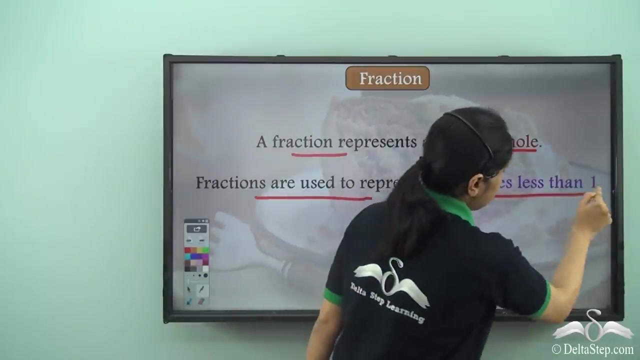 or 1 by 2 of the chocolate. So what is the fraction? a part of whole. That is, a part of whole means a part of an entire thing, So it is used to represent quantities less than one. So when I need to represent something which is less, 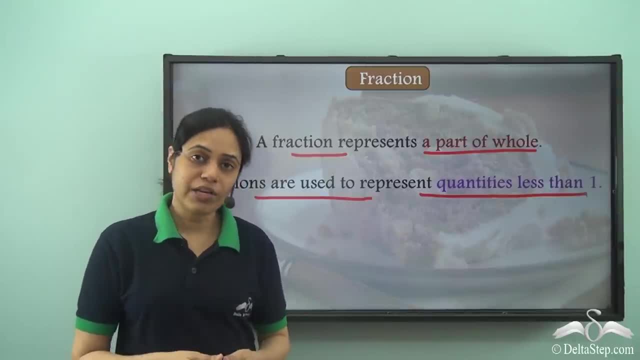 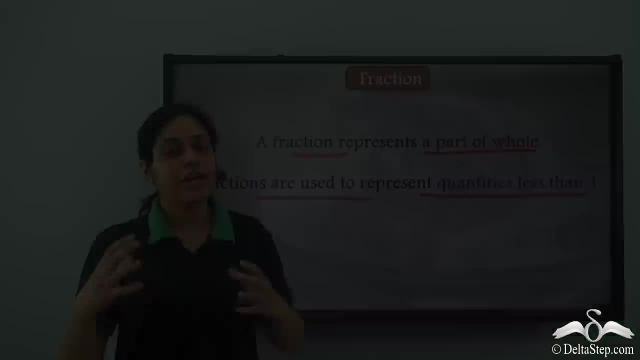 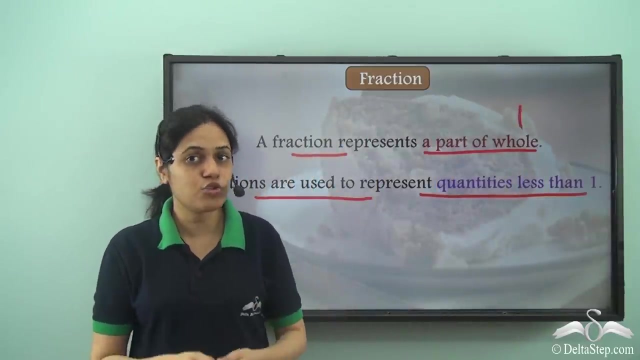 than one, I use fraction. So in the case of chocolates, each kid got less than one chocolate, So I used fraction to represent it. So it represents a part of an entire thing. So part of a whole means part of an entire thing, and it is used to represent quantities that are 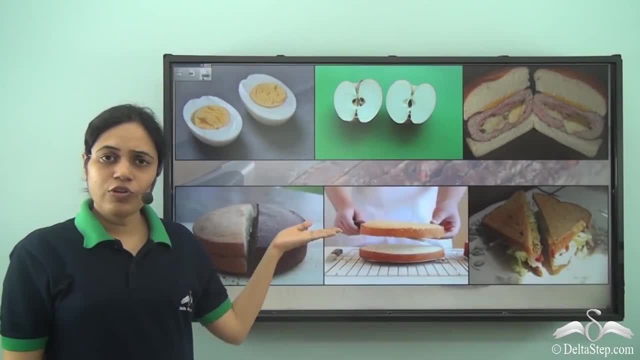 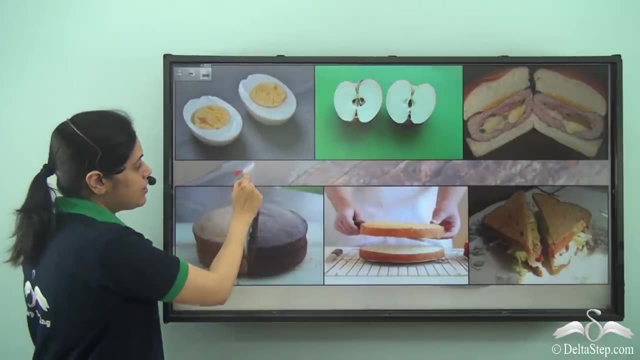 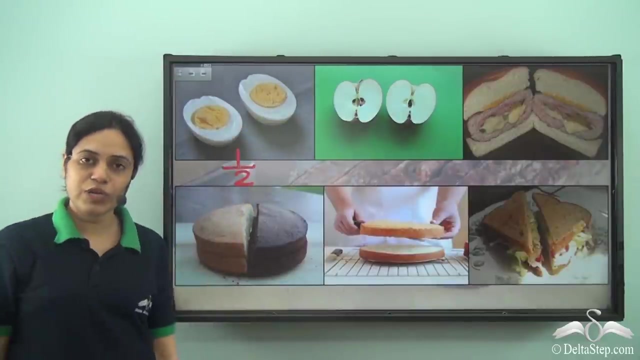 less than one. So if you look at these images now, each of the pieces of this egg, the egg is divided into two equal parts. So I write two below and if I consider each piece, it is one out of two equal pieces. So each piece can be represented as one by two. So even 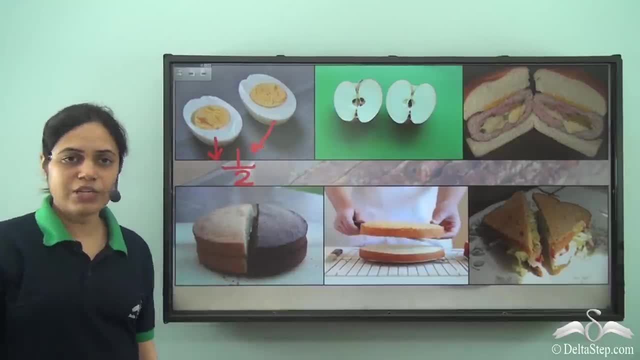 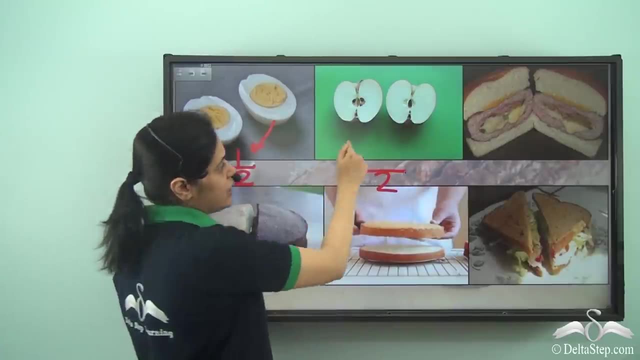 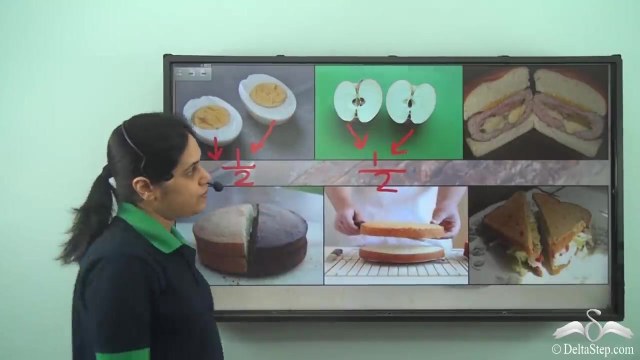 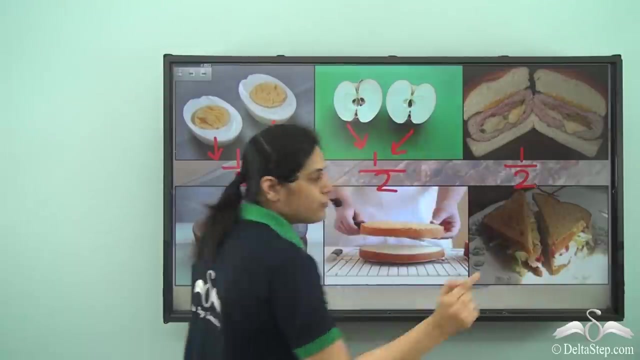 this is one by two. and this is one by two If I look at this apple. I have broken down the apple into two equal parts and each part can be written as one by two. So even this part is written as one by two. Similarly, for this burger, each part is one out of two. 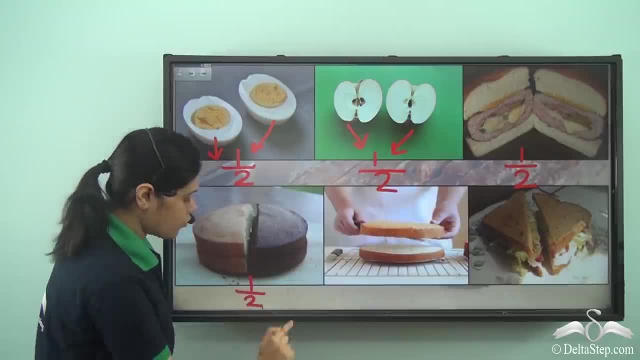 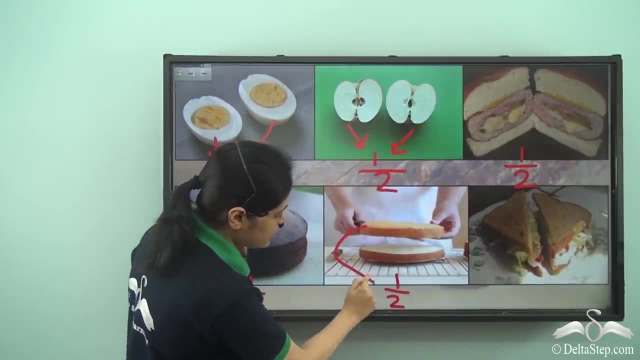 equal parts. This cake, it is one out of two equal parts. Now also we are adding that more: one out of a two equal parts. So this is single, Improving its composition. Now, this equal parts, even this cake. so one part out of two equal parts. so this part is 1 by 2,. 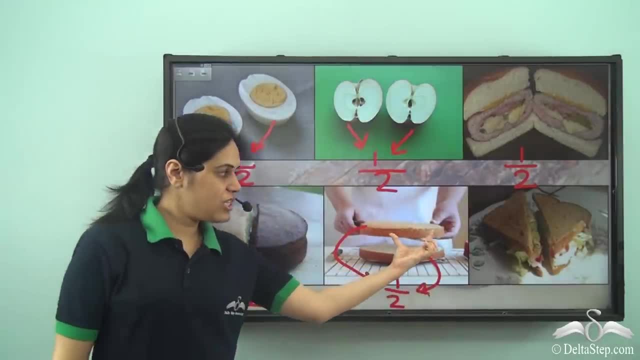 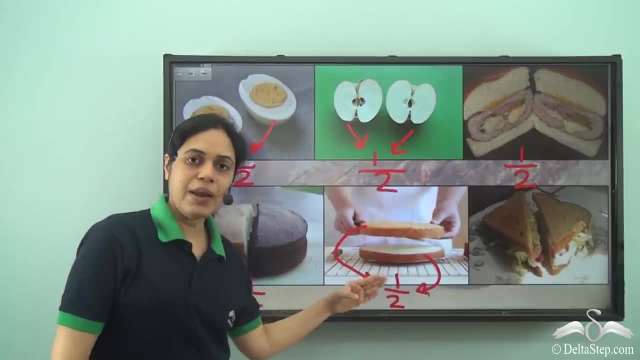 even this part is 1 by 2, so if I give you this part, will you tell me that I have given you one cake? No, you will say that I have given you 1 by 2 of the cake, even this sandwich. 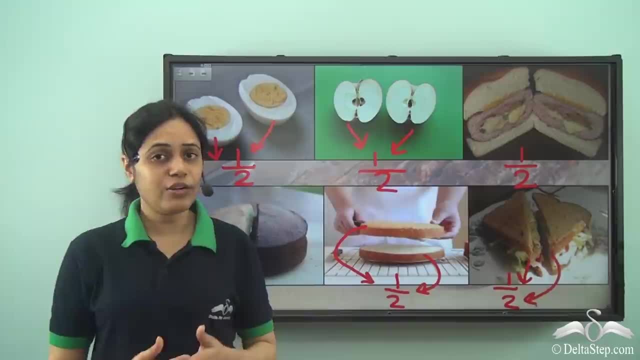 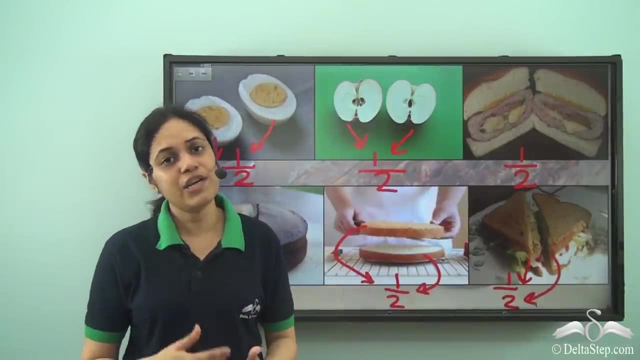 so each part is 1 by 2, so no matter what the shape is, if you divide it into two equal parts, then each part can be represented as 1 by 2, now 1 by 2 is also referred to as: 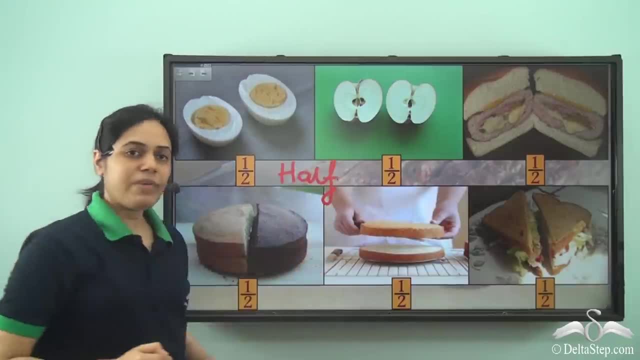 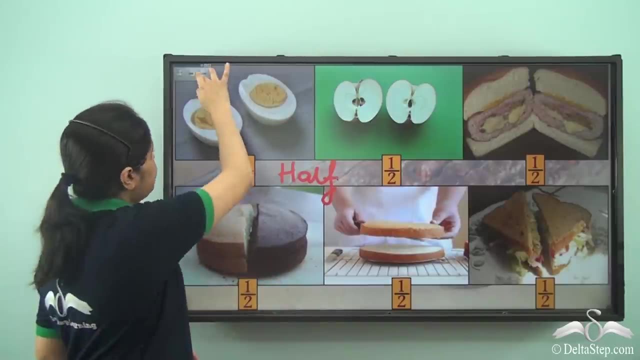 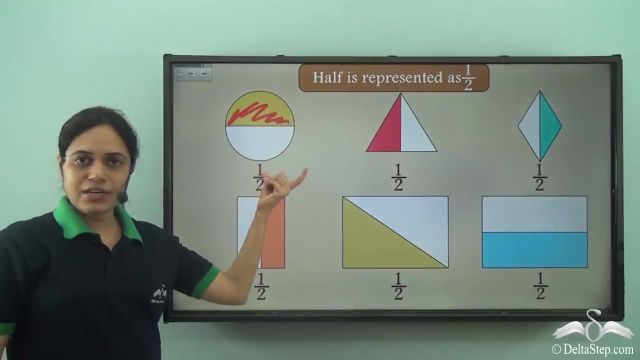 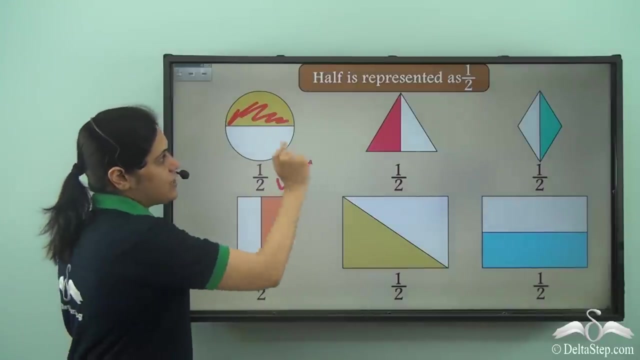 half. so 1 by 2 is called half. so each of the pieces here is half of the cake, even these images. so if you look at this coloured portion, I divide this circle into two equal parts and the coloured part is 1 out of the two equal parts, so I can write it as 1 by 2 or half. 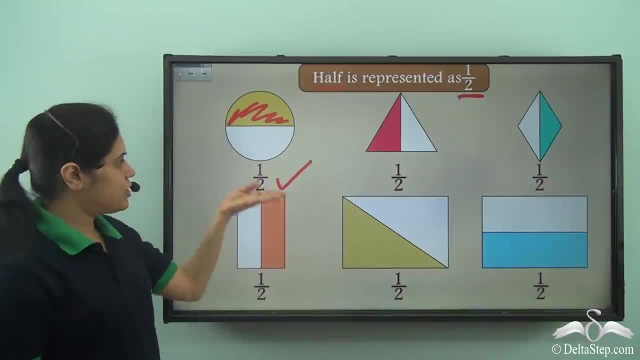 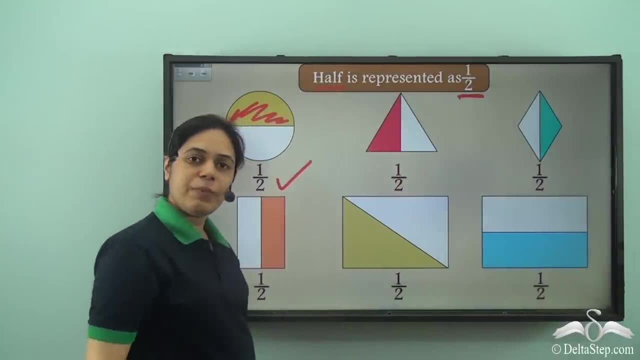 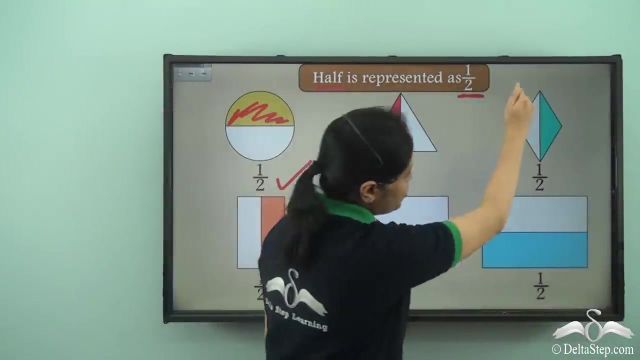 half is represented as 1 by 2, so this is half. if I look at this pink coloured portion, it is 1 out of two equal parts, so it is half or 1 by 2.. If you look at this diamond shape, it is divided into two equal parts and the shaded part is 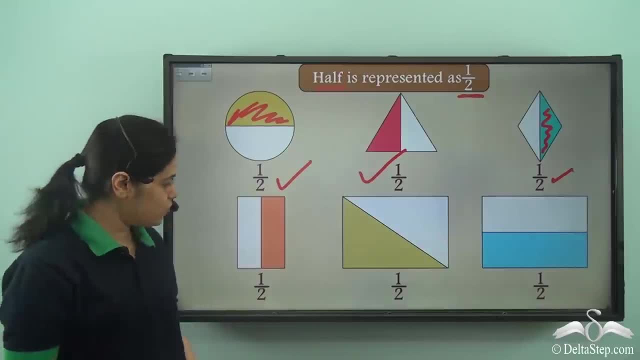 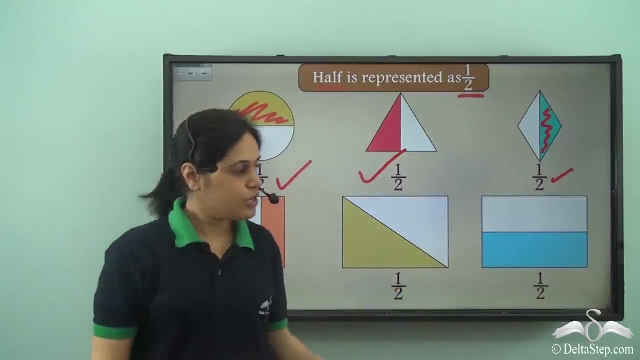 1 out of two equal parts, so I can write it as 1 by 2, even this is 1 out of two equal parts, 1 out of two equal parts and 1 out of two equal parts, so all the coloured portions. 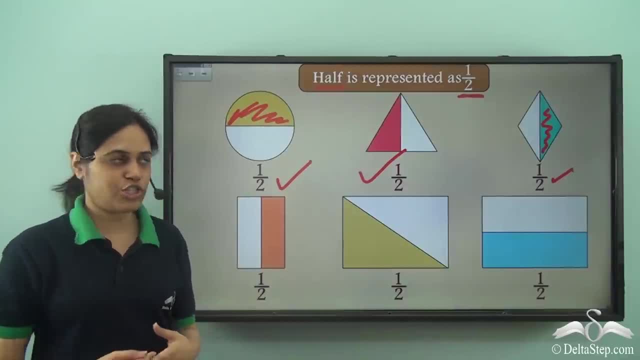 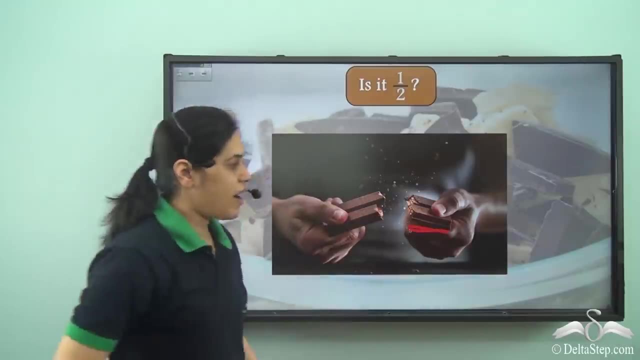 are half of the shapes or 1 by 2 of the shapes. Now this chocolate is broken into two parts. so will I say that this part is half or half of the shapes? No, you will say that this part is half of the chocolate, or whether this part is half of the chocolate. Think. 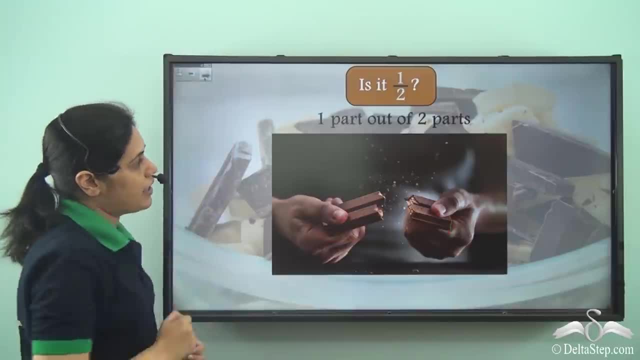 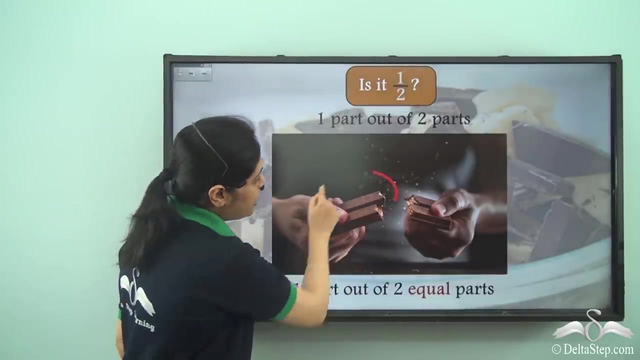 about it. it is one part out of two parts, but when can I write as 1 by 2? When I have two equal parts? so 1 by 2 is actually 1 out of two equal parts, but, as you can clearly, 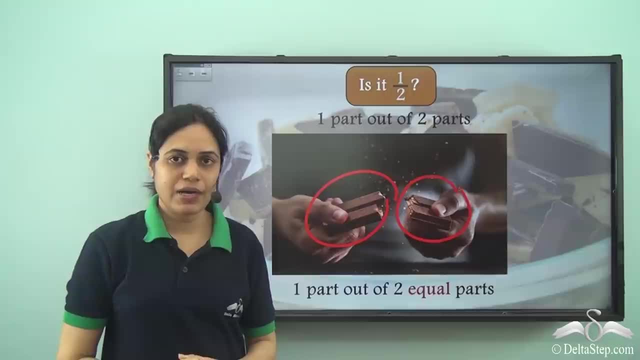 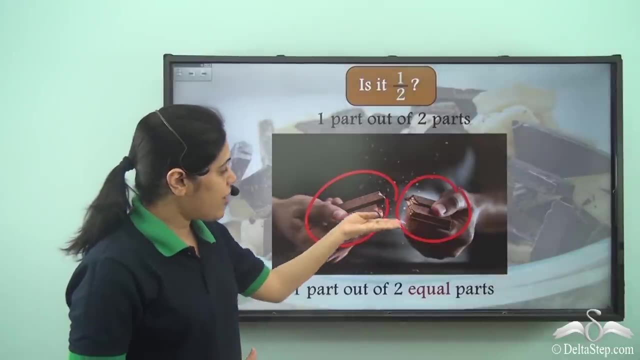 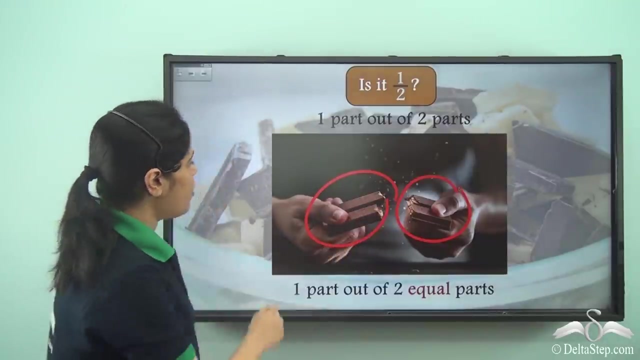 see, these are not two equal parts. This part is half of the chocolate and this part is half of the chocolate, So this is smaller than this part. So these are not two equal parts. So I cannot represent this as a fraction, because for fraction we need equal parts. So I cannot write it half, It is not. 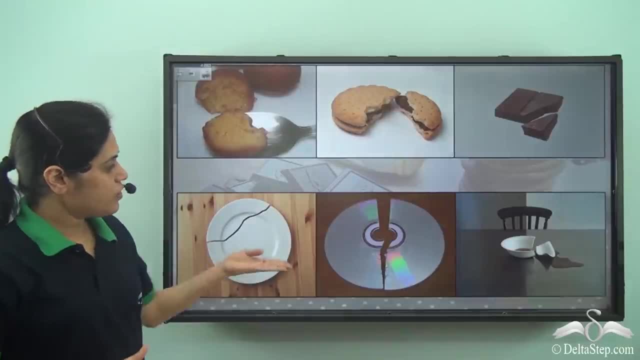 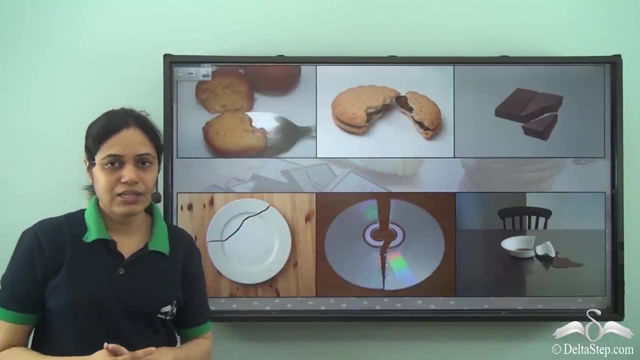 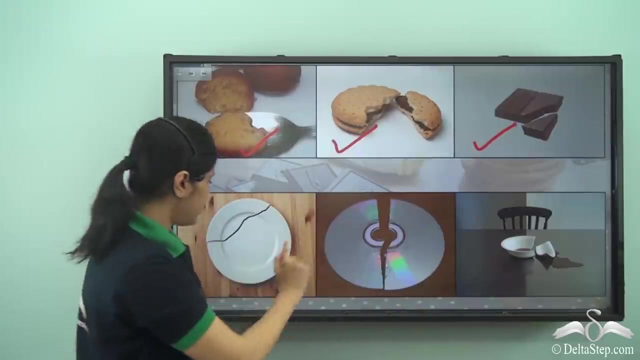 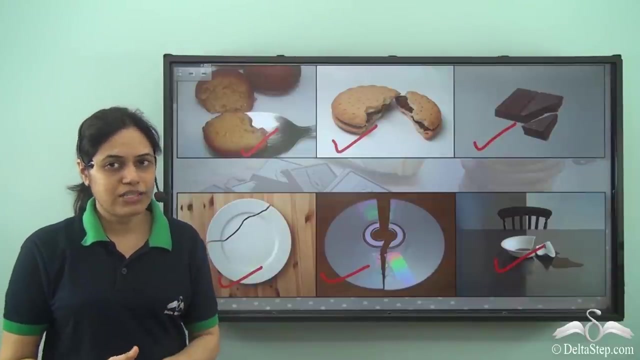 half or one by two. So if you look at all the images here, all these things are broken down into two parts, but they are not two equal parts. Be it this sweet, this biscuit, this chocolate plate, CD or this bowl, Everything is broken into two parts, but not two equal. 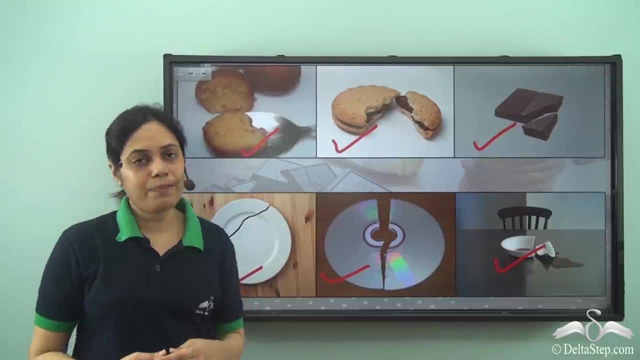 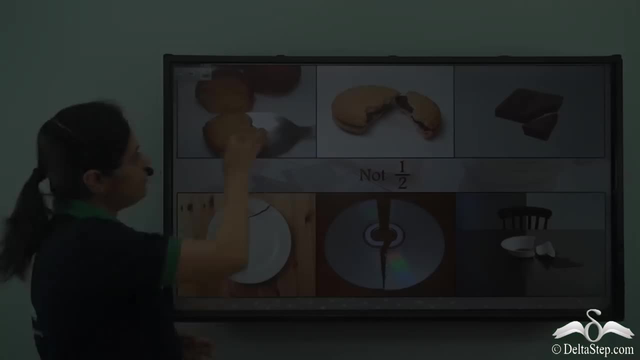 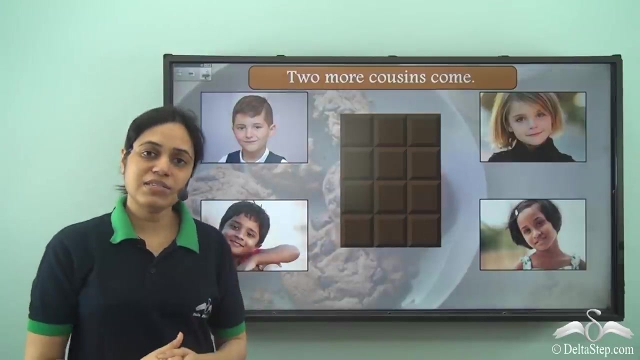 parts, So I cannot refer to one part as half. I cannot write it like this, So these are not half. Now it so happens that the day Abeer's mother bought one chocolate, two more cousins came to their place. Now what are they supposed to do? 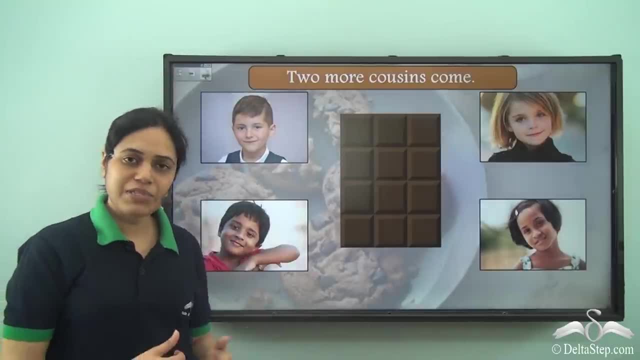 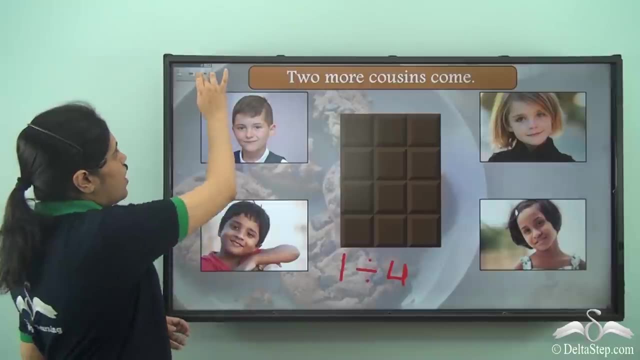 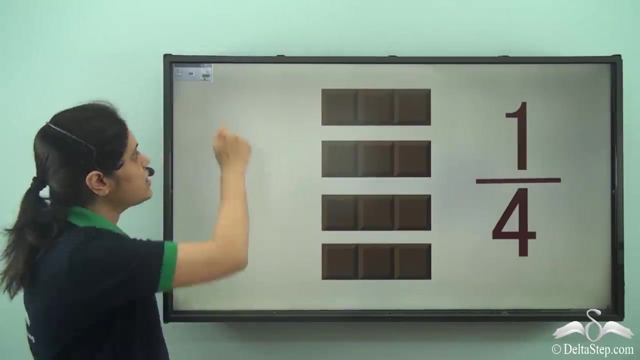 They are supposed to divide the chocolate among themselves. So this one chocolate has to be divided among four kids. So Abeer's mother took the chocolate and broke it into four equal parts, and each part is 1 by 4. So there are four equal parts, So I know. 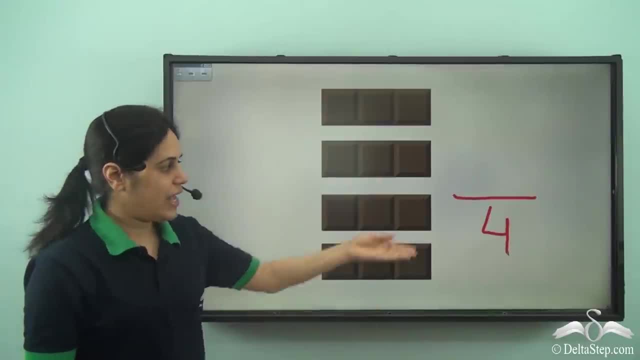 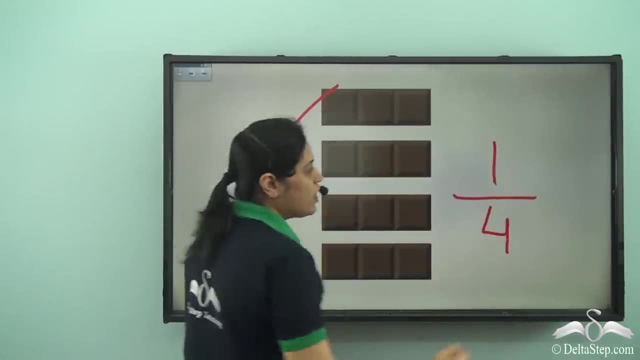 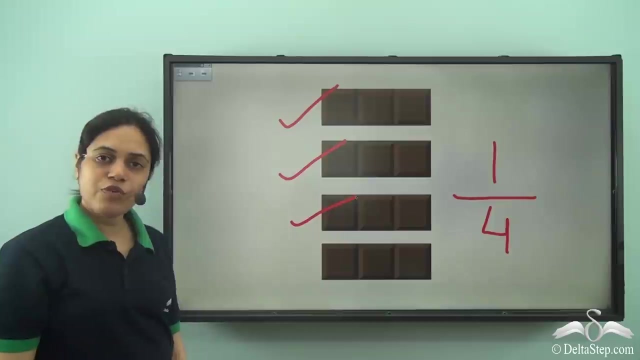 I write total number of parts at the bottom and there is a line separating and each part, that is. if I take this part, it is one out of four equal parts. Even this part is one out of four equal parts. This part is one out of four equal parts and this part is one out of four equal parts. 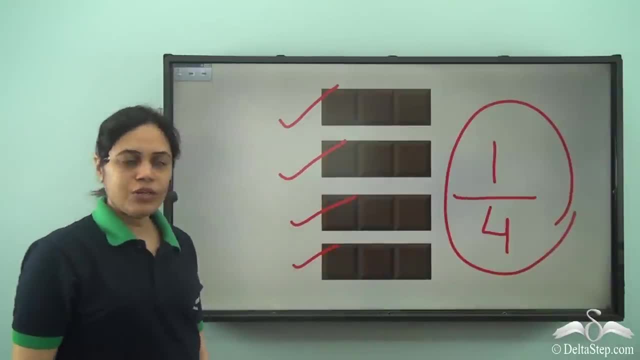 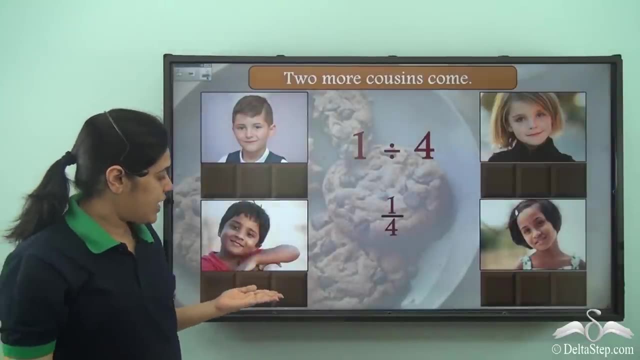 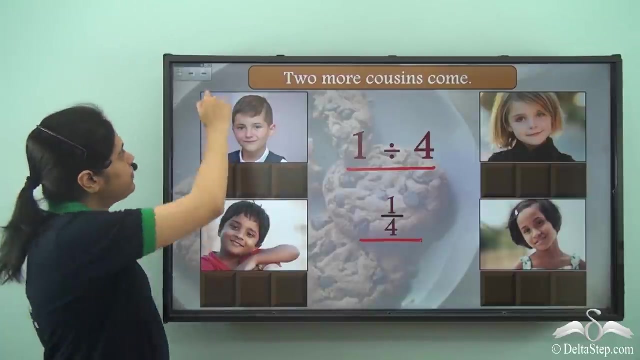 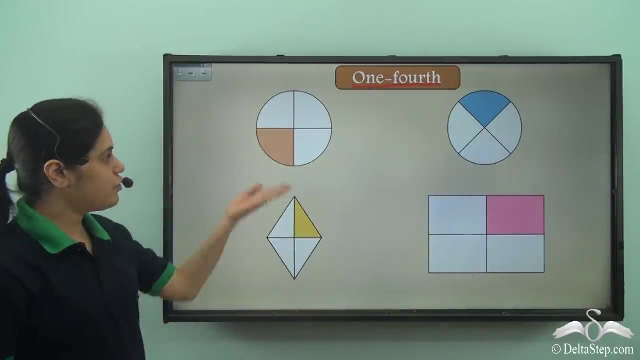 So it is 1 by 4.. So each of them gets 1 by 4 of the chocolate. So they get 1 by 4 of the chocolate, 1 by 4 of the chocolate. 1 by 4 is also called one fourth. Now if you look at this circle, 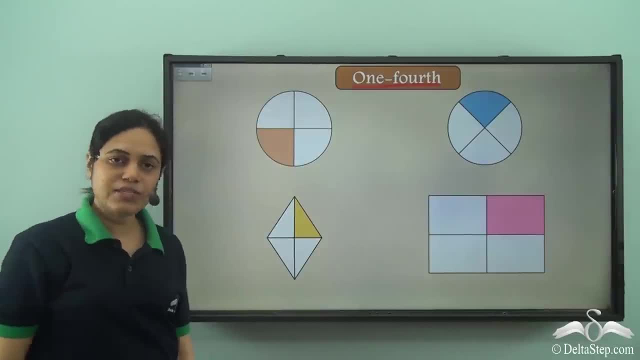 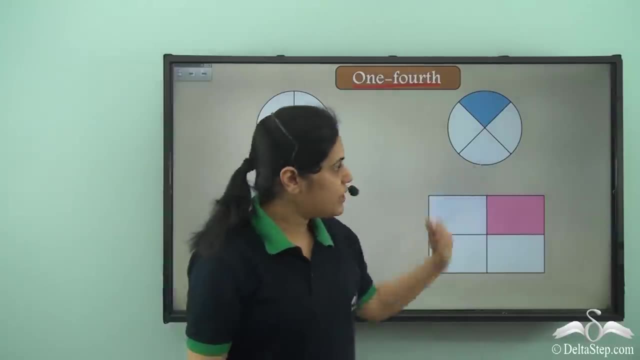 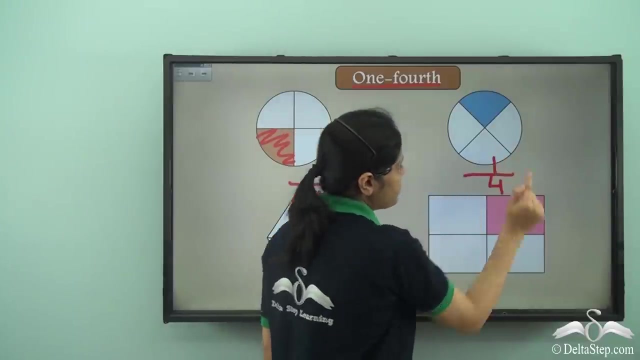 this circle has been divided into four equal parts and this shaded part is one out of four equal parts. Even this circle, it is also being divided into four equal parts and the colored portion is one out of four equal parts, So I can write it as one fourth. So remember one fourth. 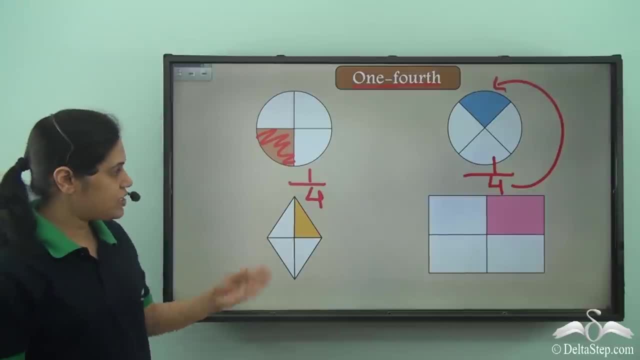 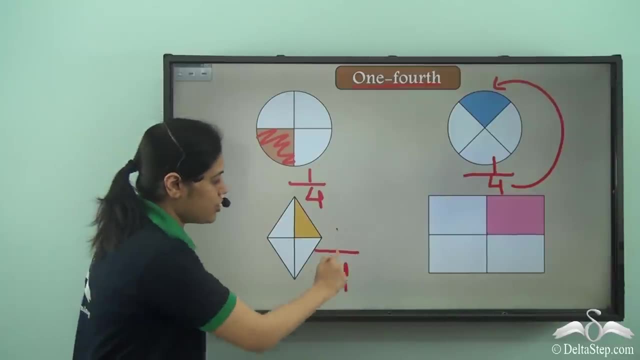 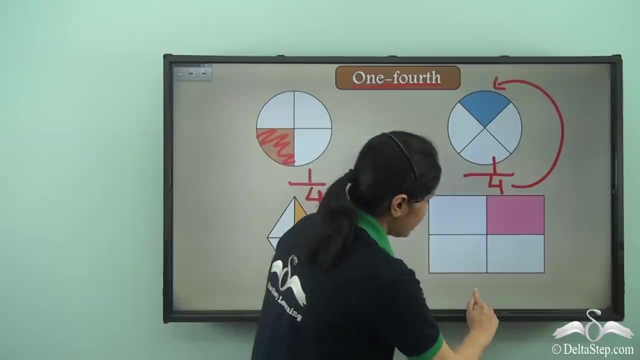 refers to this colored portion. What is this colored portion? This diamond shape is divided into four equal parts and this colored portion is one out of four equal parts, So 1 by 4.. Same for this: It is divided into four equal parts and this colored portion. 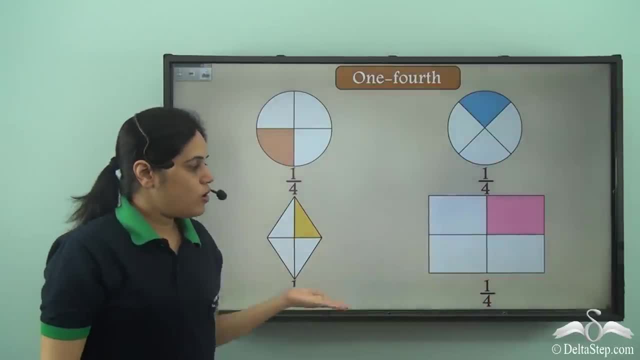 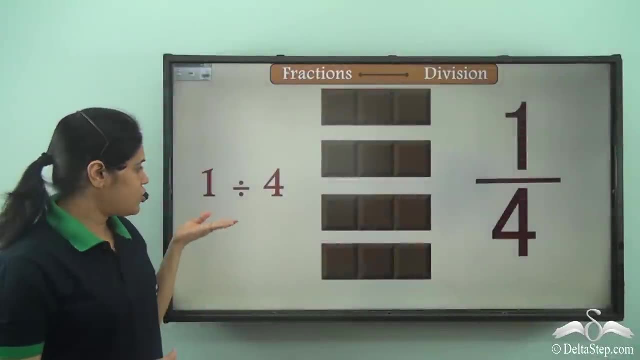 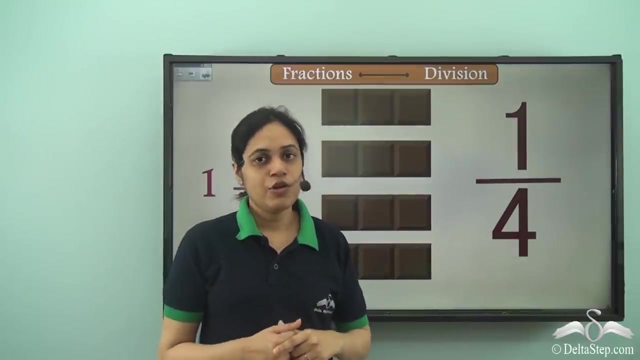 is one out of four equal parts. So all these colored portions are one fourth or 1 by 4.. Now when one chocolate was divided among four kids, each of them got 1 by 4 of the chocolate. So I can say that fractions 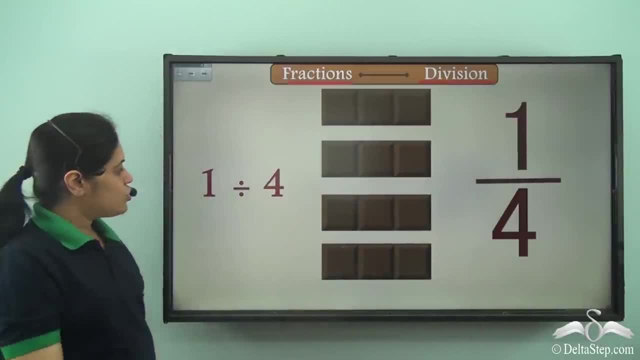 are the same as division. So if I need to divide 1 by 4, the answer is this: So 1 divided by 4 gives 1 by 4.. That is, if I divide one chocolate among four people, each of them gets 1 by 4 of the chocolate. 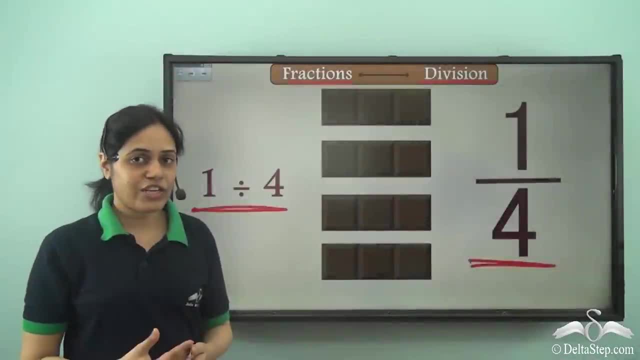 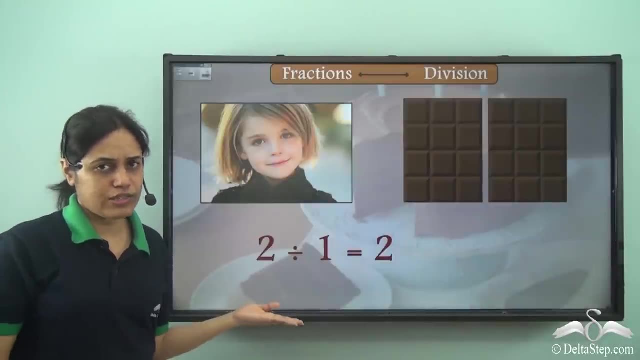 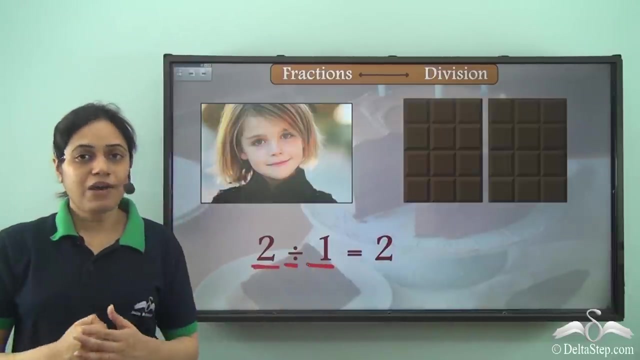 So this is the answer of division. So fractions are the same as division. So now, if your mother gets two chocolates and you are the only one present at home, So the two chocolates will be divided in one person. So it will be 2 divided by 1.. 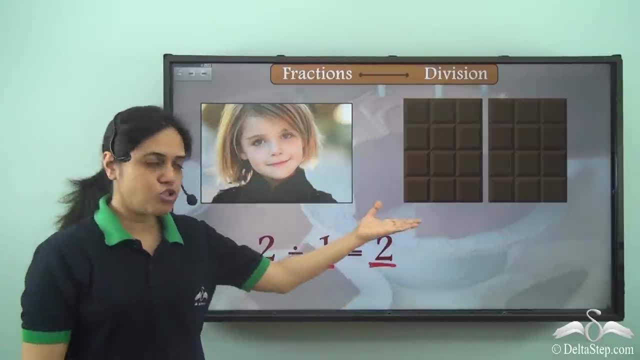 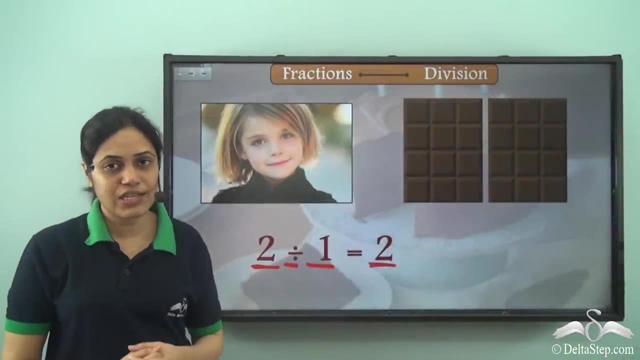 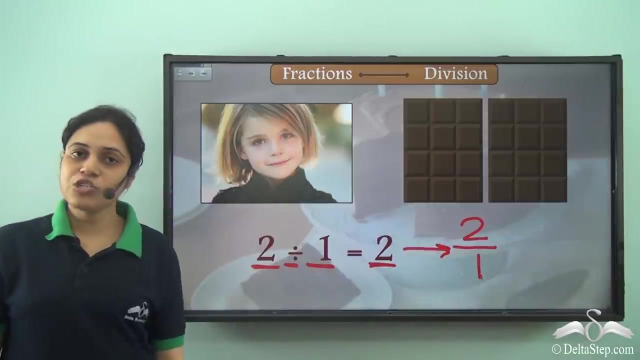 That is, you will get both the chocolates. You get two chocolates. 2 divided by 1 is equal to 2.. But now we know that division can also be represented as fraction, So 2 divided by 1 can also be written like this: 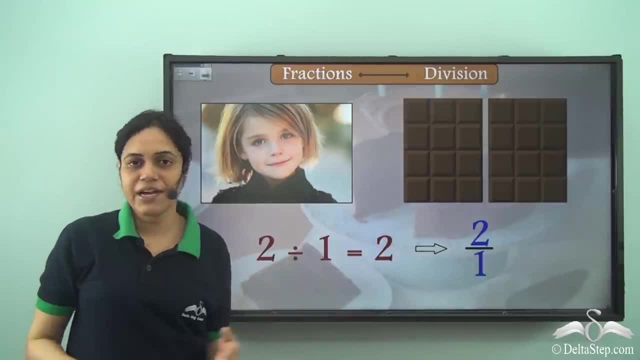 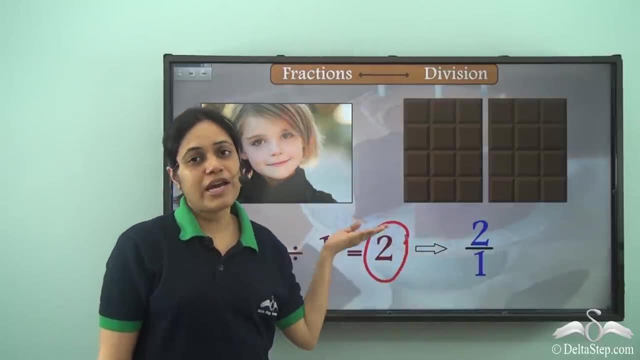 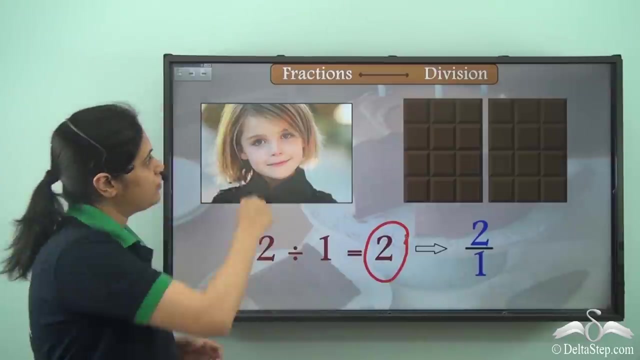 So this is 2 divided by 1.. So when I write 2, it is nothing but 2 divided by 1.. So I can write any number as a fraction with 1 at the bottom and the number at the top. So what are fractions? 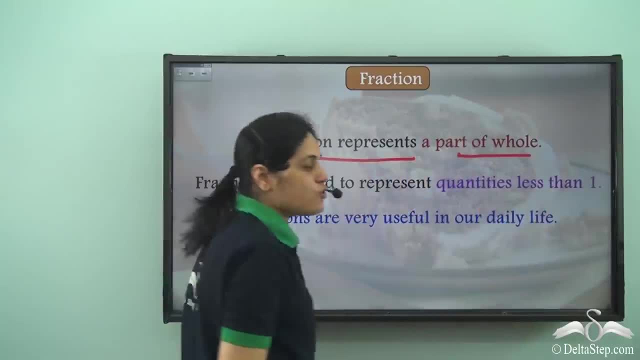 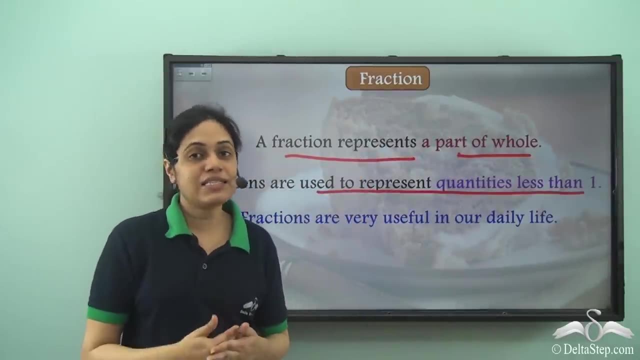 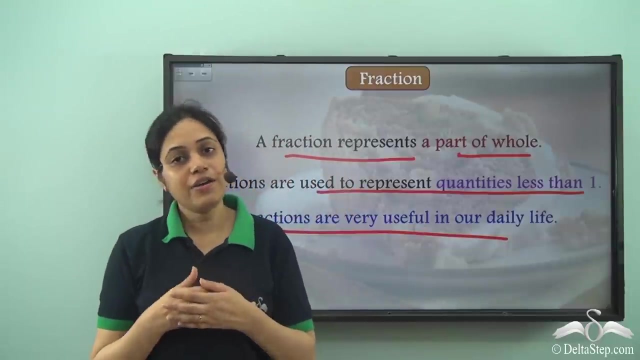 Fractions represent a part of whole, That is, they are used to represent quantities less than 1.. That is, something less than 1 is represented using fractions, And fractions are very useful in our daily life. So fractions are same as division. In fact, division can be represented. 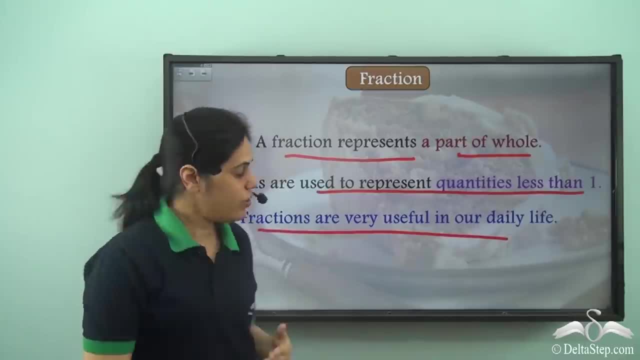 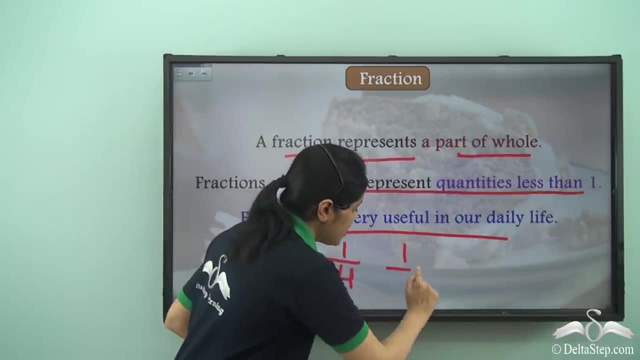 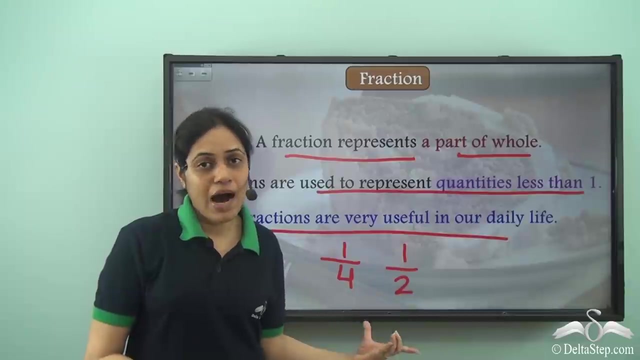 using fraction. So 1 divided by 4 can be written as 1 by 4 using fractions. 2 divided by 2 can be written as 1 by 2 using fractions, And these quantities are all a part of an entire thing. 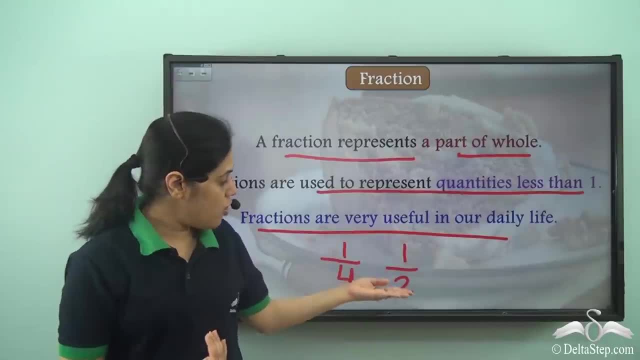 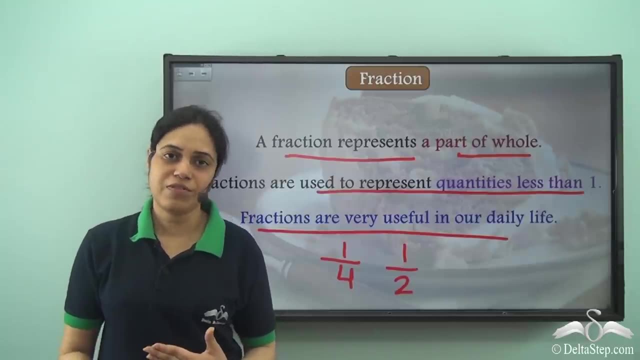 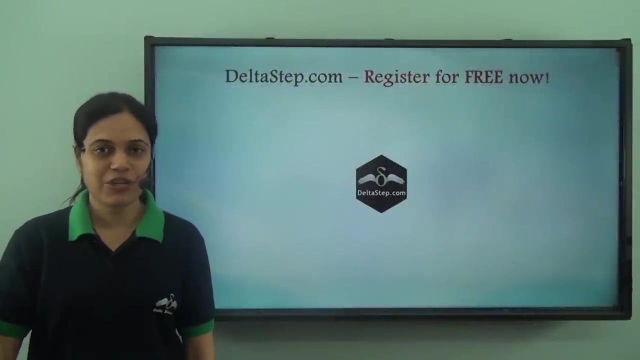 or a part of whole. So fractions are used to represent part of a whole, That is, they are used for quantities less than 1.. So practice them till you get comfortable with them. If you like this video, then subscribe to our channel. 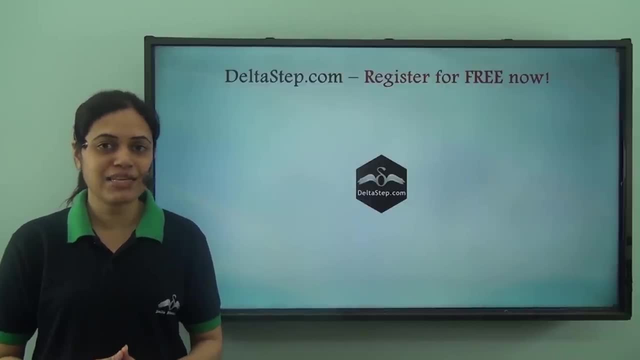 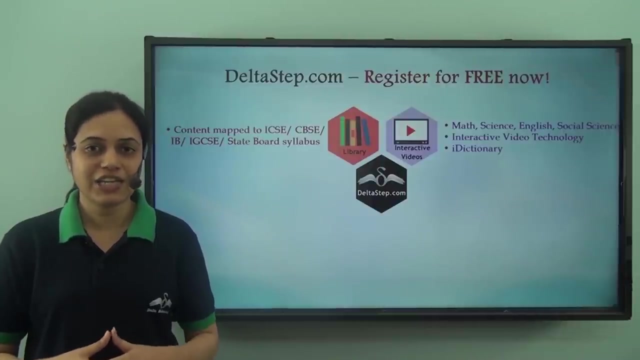 You can also register for free at deltastepcom to get all the learning resources as per CBSC, ICSC, IB, Cambridge or any other curriculum. Over 5000 amazing lectures on Maths, Science, English and Social Science. Our unique interactive video technology: